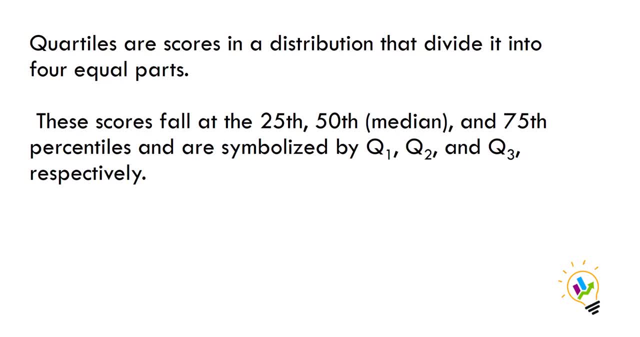 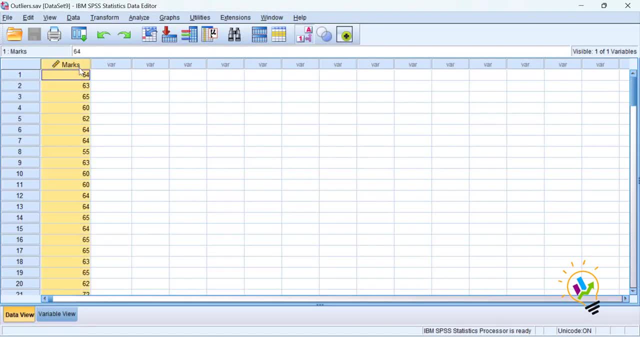 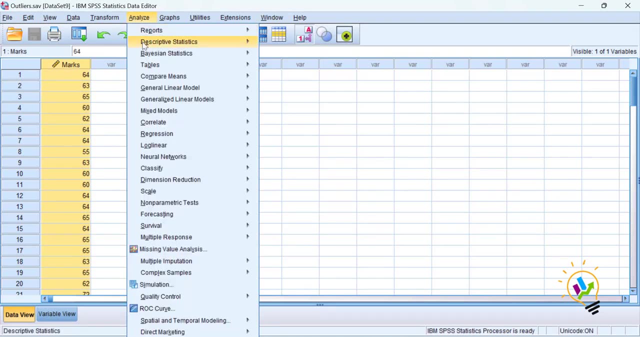 and are symbolized as Q1, Q2 and Q3 respectively. Let us see with the help of an example- This is a scale data marks. and now let us see the distribution of this data into quartile. For that, analyze descriptives, frequency In this, select marks and click ok. 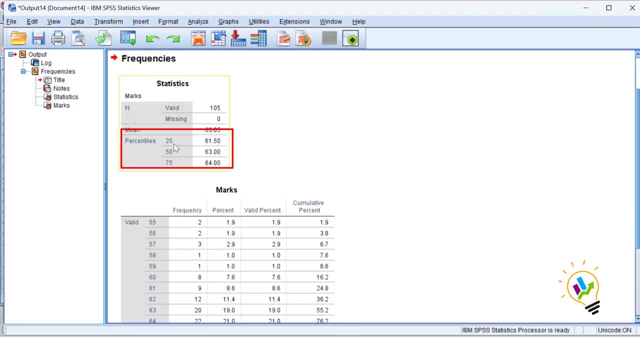 Now we are going to get the percentiles. 25th percentile is first quartile. Its value is 61.5.. 50th percentile is 63. This is second quartile, and 75th percentile of the data distribution is 64.5.. 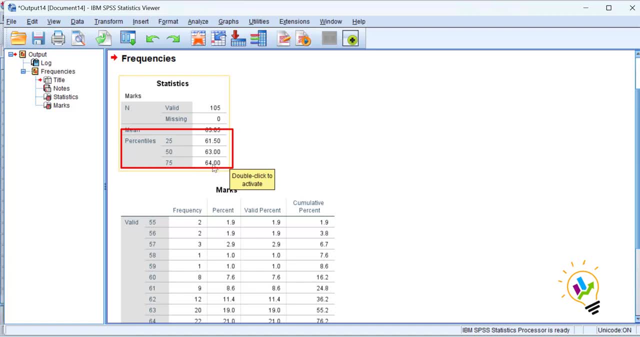 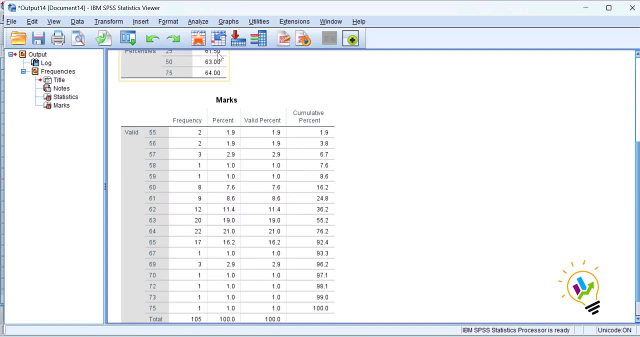 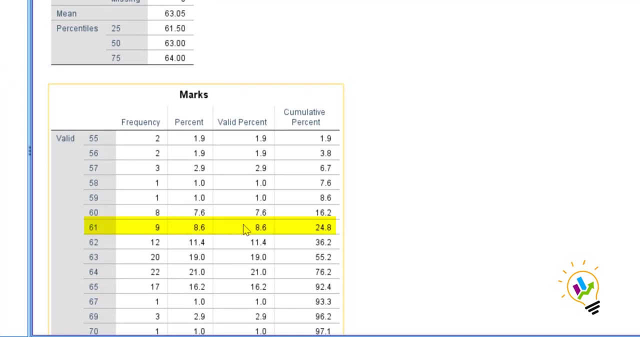 This is 64.00.. This is 75th percentile, which is called a third quartile. If you see the data distribution here: 61.5.. 61.5 is a first quartile, means this point above 61 point. So till here it. 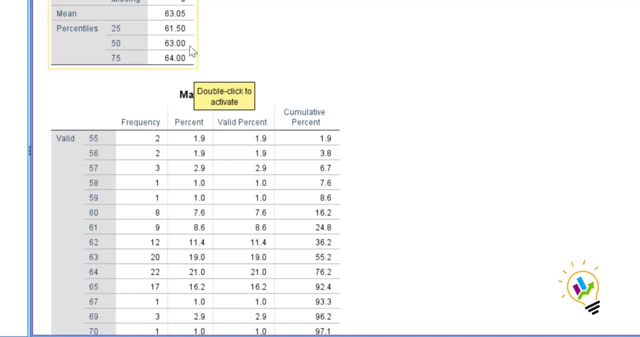 is all called as first quartile, and 63, this is called this range is called as median, which is 50th percentile, And 64. This is called as a third quartile, So 61. This is the first quartile, the distribution. 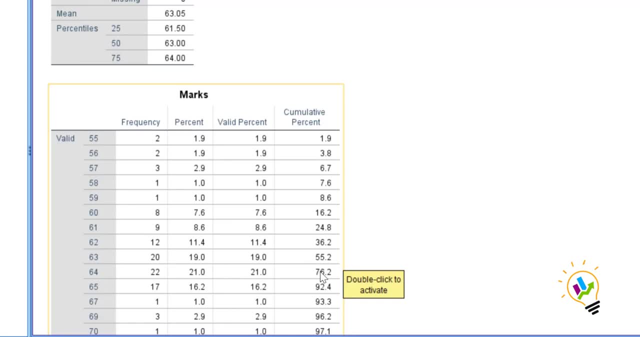 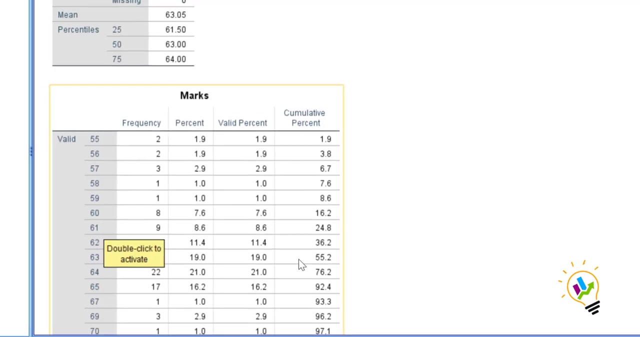 This is second quartile and this is the third quartile. that difference between first quartile, two, the third quartile, Is called as inter-quartile range, so 64 minus 61.. This is three. This three is called as inter percentile range. 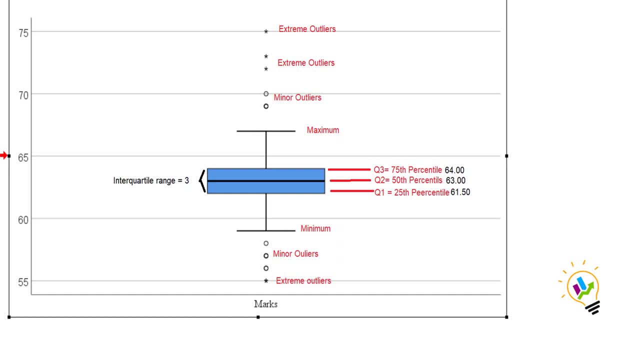 now, if you see this distribution, we will understand. this is a box plot. here we can see the first quartile is 25 percentile- okay, 61.5. this is the first person, and the second quartile is 50th percentile- 63. this is a range and this is the third quartile range and the minimum and 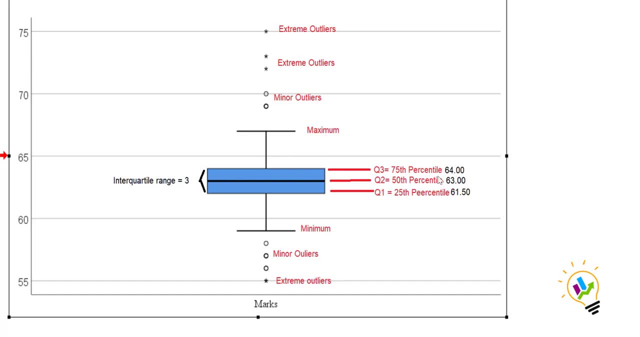 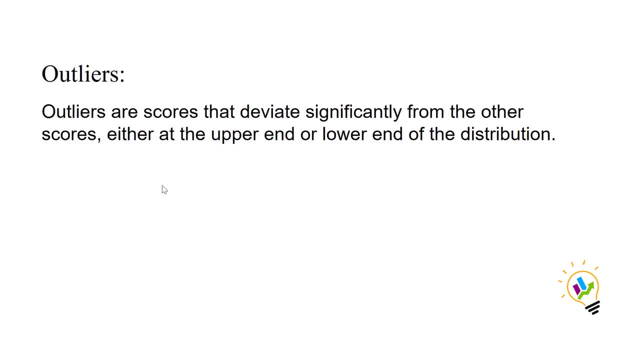 this is maximum score. the difference between first quartile to third quartile is called interquartile range. now let us see what is outliers. outliers are scores that deviate significantly from the other scores, either at the upper end or the lower end of the distribution. 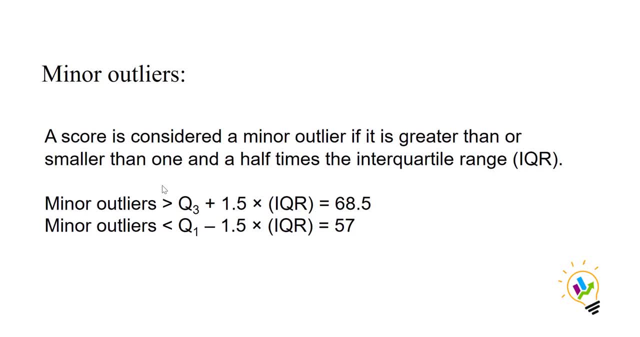 there are two type of outliers: minor outliers and major outliers, that is, extreme outliers, minor outliers. a score is considered a minor outlier if it is greater than or smaller than one and a half times the quartile range. that is, minor quartile is always calculated with quartile 3 plus 1.3 into interquartile range. 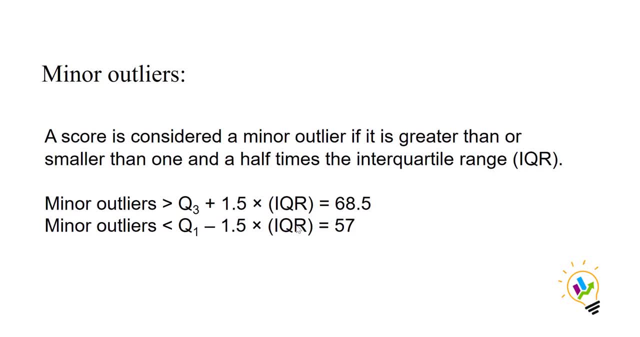 in our calculation it is 68.5, and minor quartile, which is less than is quartile 1 minus 1.5, into iq or interquartile range, which is going to come as 57. now if you see the extreme quartile range. 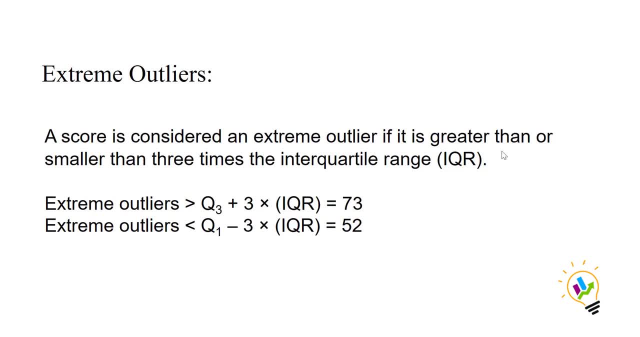 a score is considered as extreme outlier if it is greater than or smaller than three times the interquartile range. extreme quartile range: you can see: q3 plus a 3 into iq or 73. extreme quartile range: q1 minus 3 into iq or 52. now if you see the diagram, 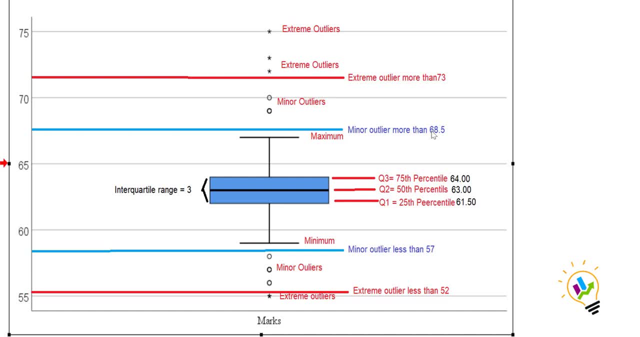 the values which are more than this value, that is, 68.5. this is symbolized as a circle. you can see these are minor outliers and values which are more than 73, which are symbolized as a star marks. this is extreme outliers when you come to lower bound, the values which are 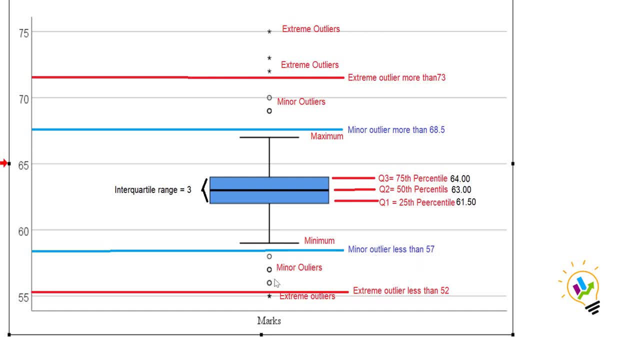 less than 57. these values are called as minor outliers, shown as the circles and the values which are less than 52, which has shown a star mark. this is extreme lower outliers. so these are outliers: extreme outliers at the extreme points and minor outliers close to the outlier. 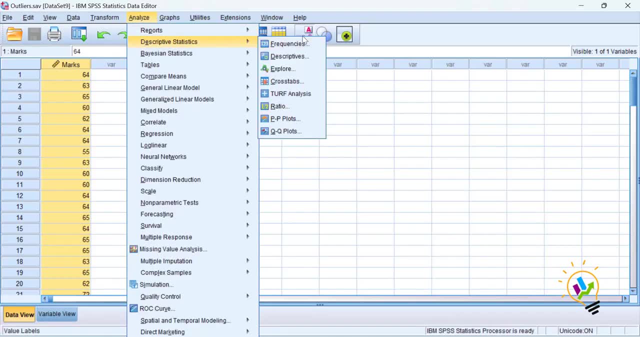 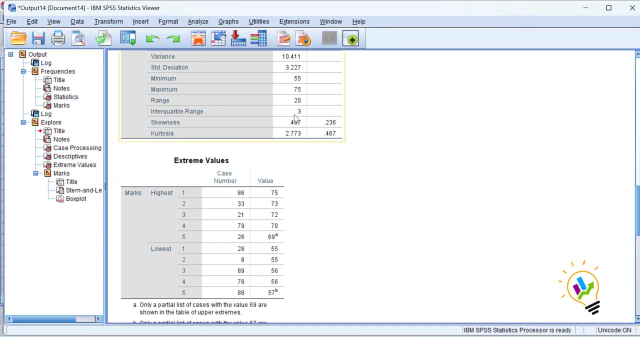 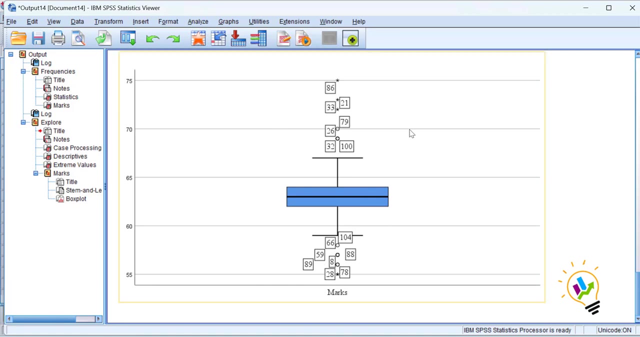 range example, analyze descriptives and in this, explore. if we take marks and click ok, we can see interquartile range is three and if you see the diagram, this is a diagram where we can see, uh, the extreme outliers and minor outliers which are distributed and these numbers are case numbers. you can see in the data. 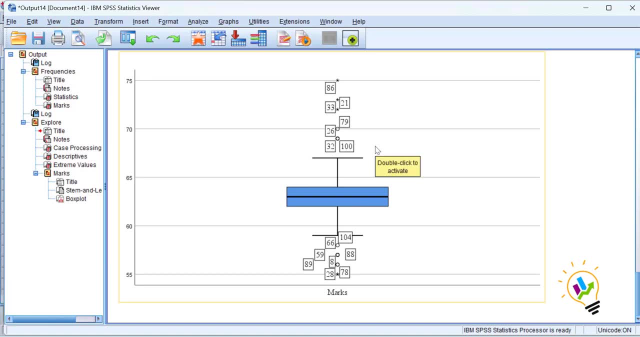 these are the case numbers, so i wish you understood what are outliers and i wish this video will be useful for your research. thank you.